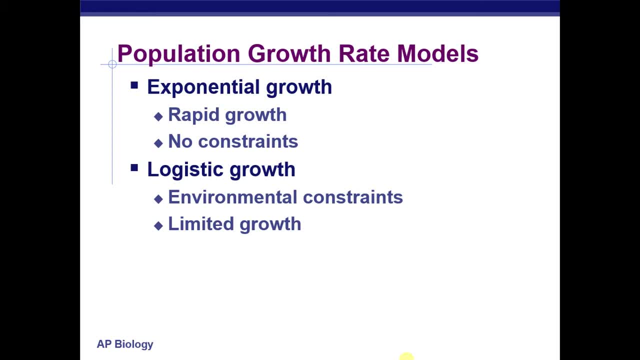 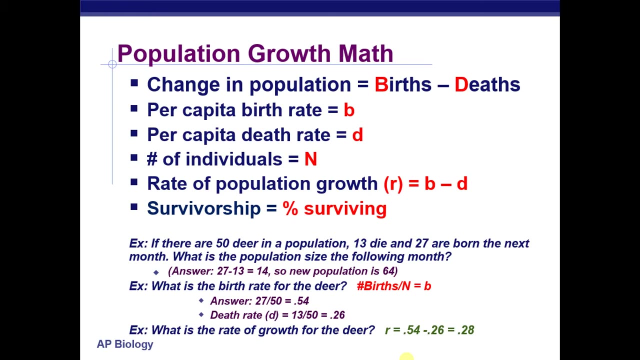 of each. We'll look at the formulas, because the formulas for each growth model are on your AP Biology formula sheet, So you'll need to use them to do some helpful calculations. So, in general, if we want to understand the change in a population size, we take the births minus the deaths. Remember last? 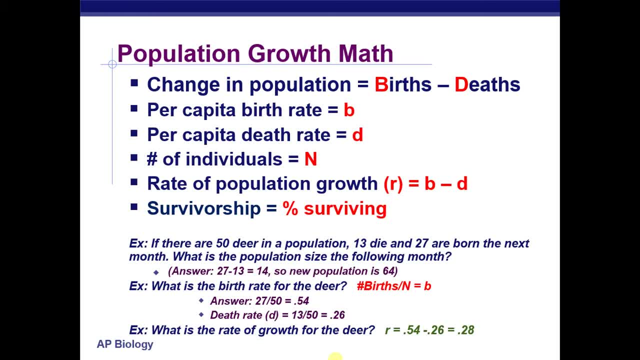 time I said, in most situations we can take immigration and emigration to cancel out. Now there's many more advanced and more complicated models we could make when those contributions aren't zero, but for our class we'll assume that they cancel out and we'll focus on births. 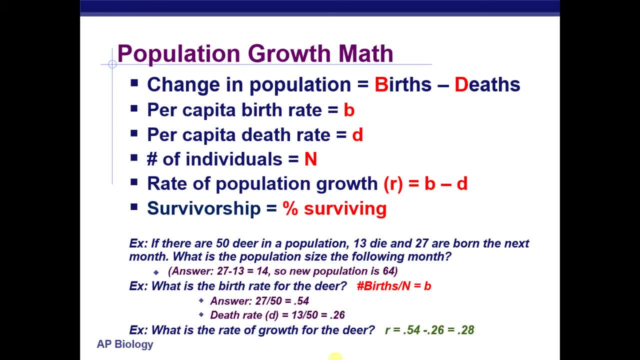 minus deaths. So we can also then take the births minus deaths. So in total number of births, in total number of deaths, And we can find what's called the per capita birth rate and the per capita death rate, the little b and little d. So little b is just when you take all the births. 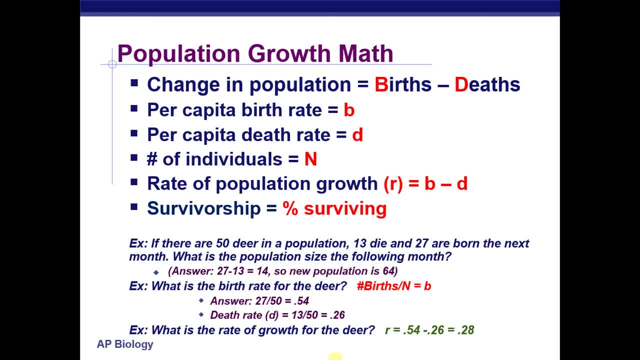 in a population and divide it by the number of individuals, or n. And similarly little letter D is when you take all of the deaths in a population and divide it by the number of individuals, n. Why would we? we would want to do that is so that we. 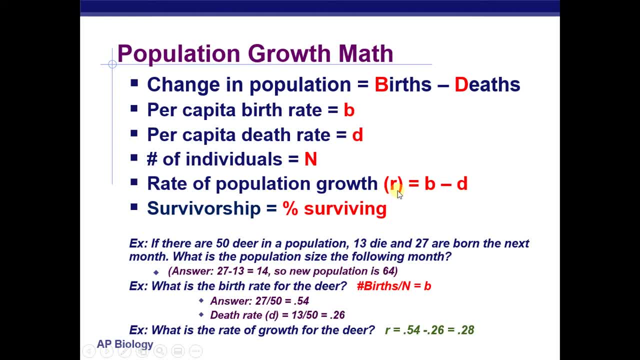 can figure out the rate of population growth R. R is what's going to be really important in these models, and R is the per capita birth rate minus the per capita death rate. so little b minus little d, right, that'll be important. and then, lastly, survivorship is just the percentage of the total population. 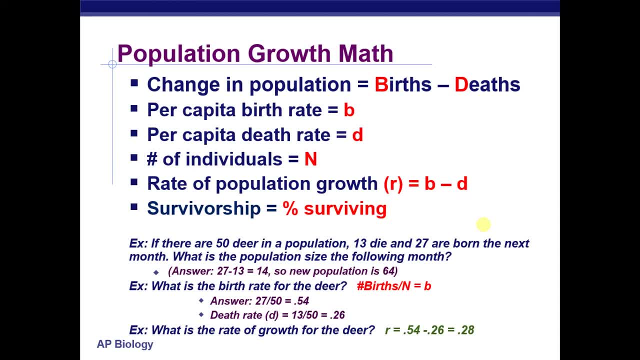 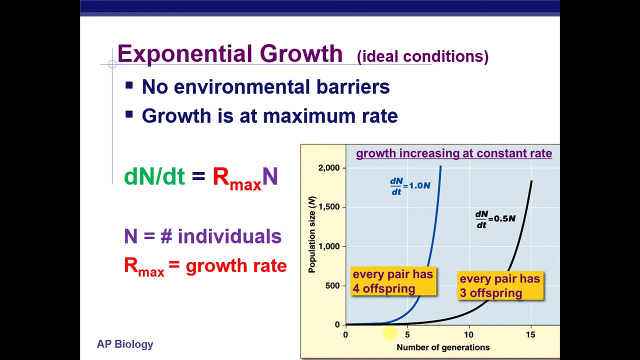 surviving over a specific period of time. So down here at the bottom you can take a look at a few examples about how we would calculate little b and little d, and then also how we would calculate R. So first we'll look at exponential growth, which is what would happen in. 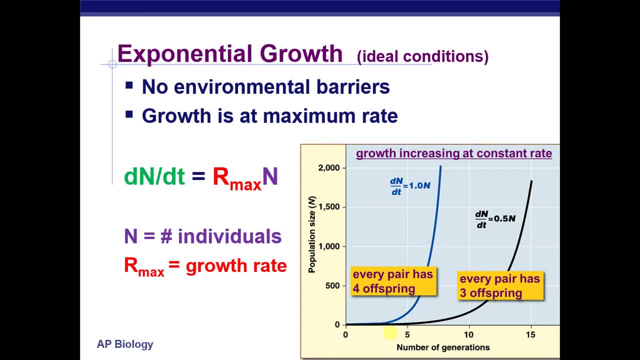 ideal conditions, and exponential growth is a model we can use that assumes there's no environmental barriers, so there is no limitation of resources, and that the population is going to grow at a maximal rate. And so werd We have in this slide the equation for exponential growth, where we have the differential of n. 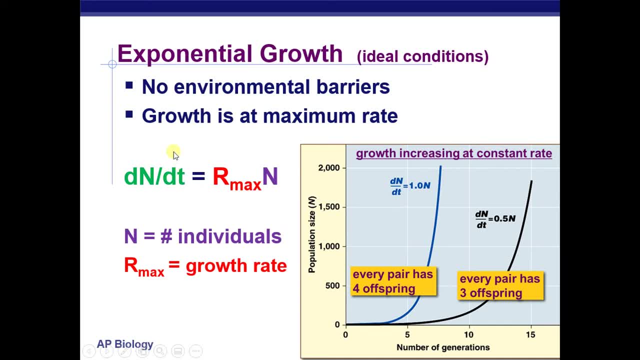 with respect to t. So, for those of us who have taken calculus, this is the derivative of n with respect to t or, if we haven't, simply the change in the population size over time. The change in the population size over time is equal to the maximum growth rate times. 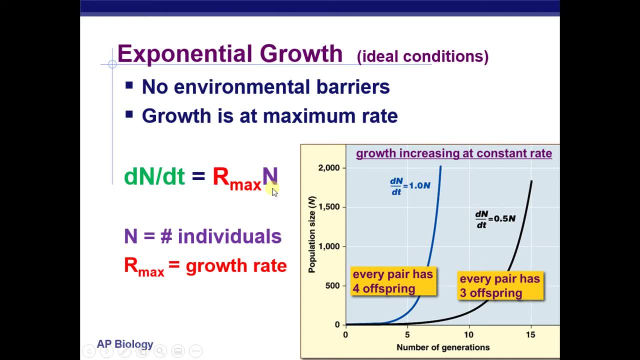 the number of individuals. So if we look at the graph, it's going to look something like this, And here you can see how two related graphs would look if we change with the on the graph. So this is what our max value is. 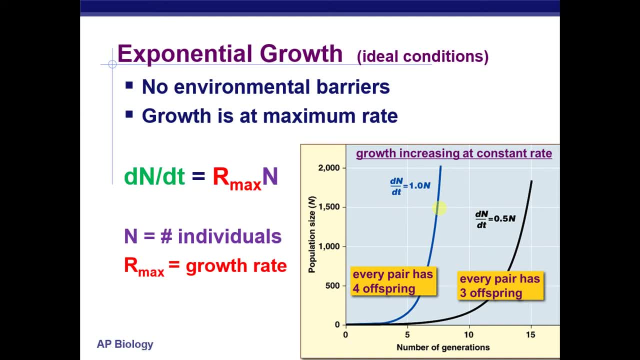 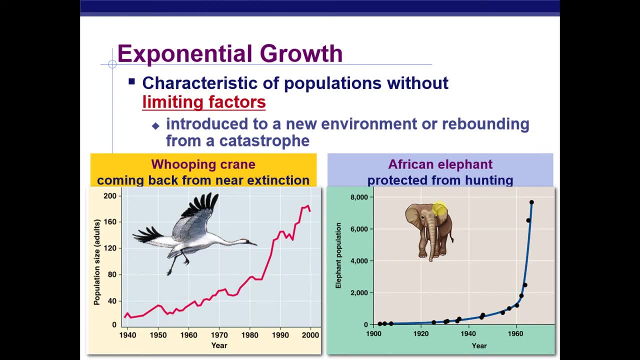 So pretty straight forward. So exponential growth is a characteristic of population without limiting factors. So there aren't any factors from the environment, like need necessary resources, that limit how fast the population can grow. And this is actually pretty accurate when you're looking at a species. 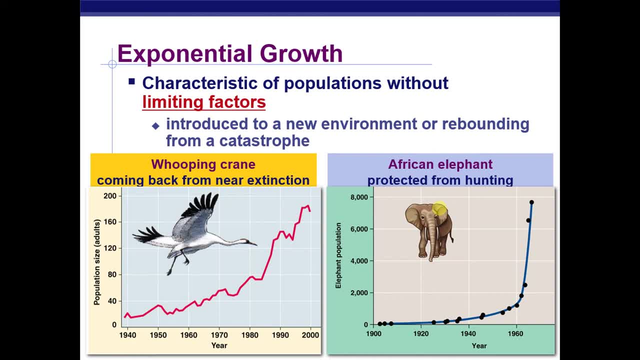 That's introduced to a new environment or has, but is rebounding from a catastrophe where their population slices shrank exponentially. So, as an example, the whooping crane coming back from near extinction, Modeled by an exponential growth rate. And once the African elephant was protected from hunting- exponential growth rate. 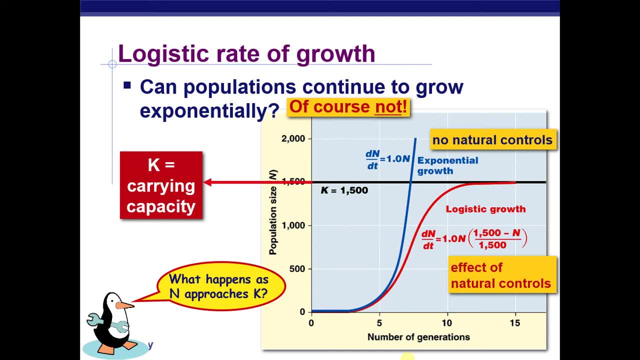 Now, populations cannot continue to grow exponentially Because each- or we'll say every- ecosystem can only support so many individuals of a given species because of limited resources. So what we do with the exponential growth rate is we limit, is we introduce the idea of K carrying capacity? 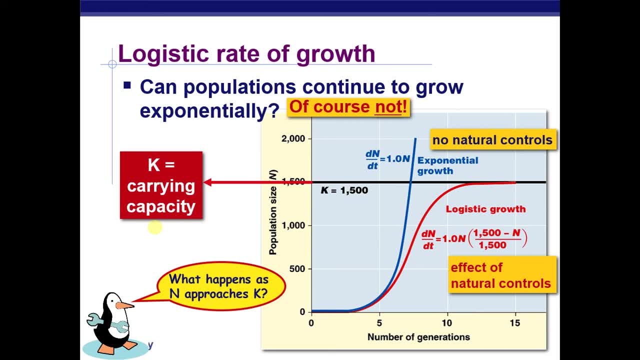 So carrying capacity is the maximal number of individuals that have a given species, That is, can be supported by the resources in a given environment. And so we introduce carrying capacity and we change our exponential growth rate formula so that the closer the population size gets to the carrying capacity, the more slowly 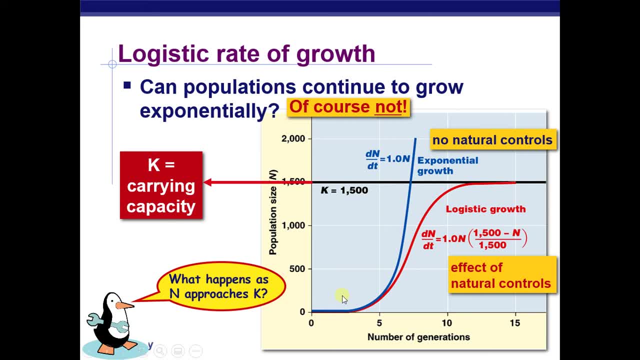 the population is going to grow And that's why on this graph, the blue line represents exponential growth and the red line is logistic growth. And that's why on this graph, the blue line represents exponential growth And you can see how the red line starts out exponentially. 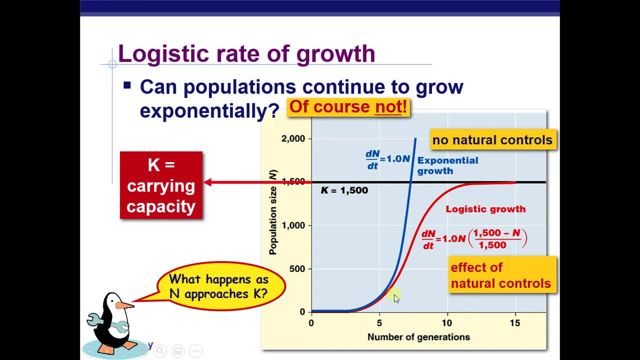 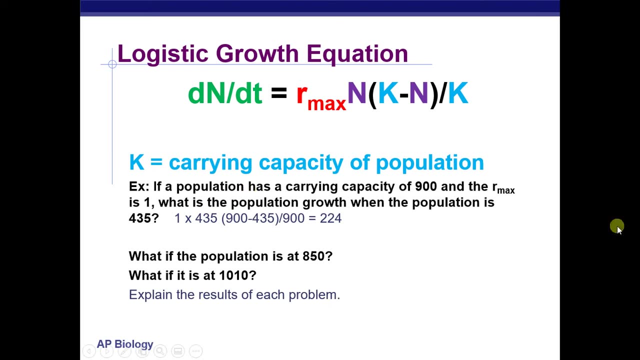 But the closer it gets to the carrying capacity, this black line, the more slowly the population starts to grow. So let's look at that equation a little bit more closely. So look at, it's very similar. We have the differential of the population with respect to time, the change in the population. 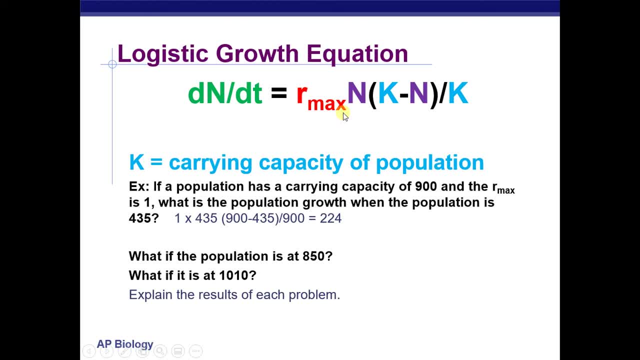 size over time equals our max times n, And look here, This is the same as the exponential growth rate. But then we have this other factor that contains the carrying capacity. Carrying capacity minus population size, divided by carrying capacity. What this last term does is the more closely 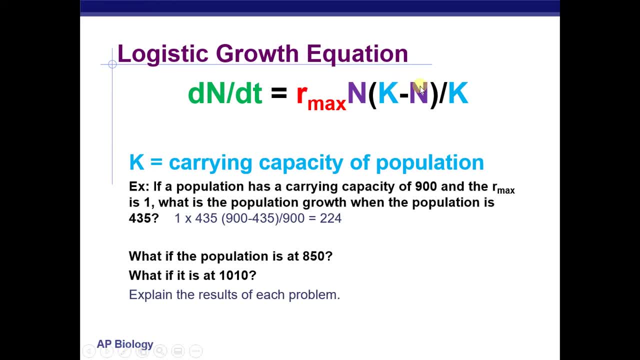 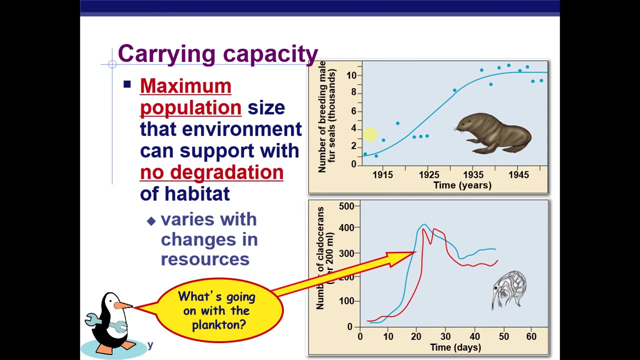 the number of individuals get to the carrying capacity, this term approaches what this term approaches: zero. so the rate of growth slows down the farther away the number of individuals is from the carrying capacity. this term approaches one, and then it just becomes the exponential growth model. all right, so, like we said, carrying capacity is the maximum population size. 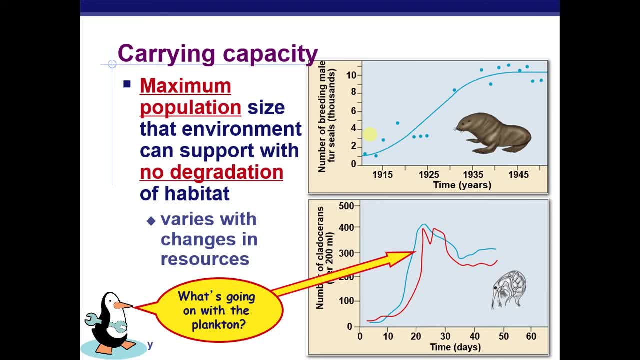 that the environment can support without any habitat degradation, and it varies with changing resources and time of year and states of the environment. so look at the number of fur seals and how they approach their carrying capacity, and the number of plankton seals and how they overshoot their carrying capacity, and so there's way more than the environment can. 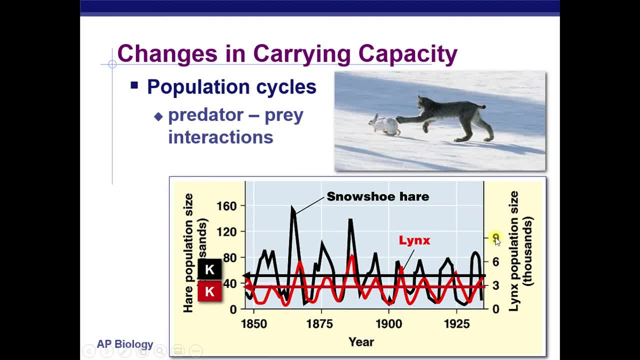 support and kind of crashes like this. so populations usually oscillate around their carrying capacity, won't have a nice asymptotic approach like with the fur seals. if you look at here we have kind of like a boom and bust model where with these predators preys they go away and overshoot their carrying capacity and then crash below it and up and down. 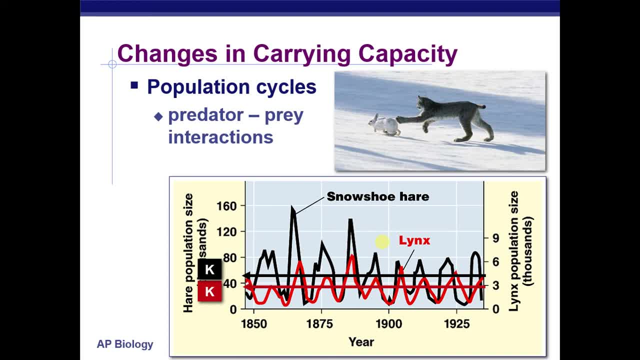 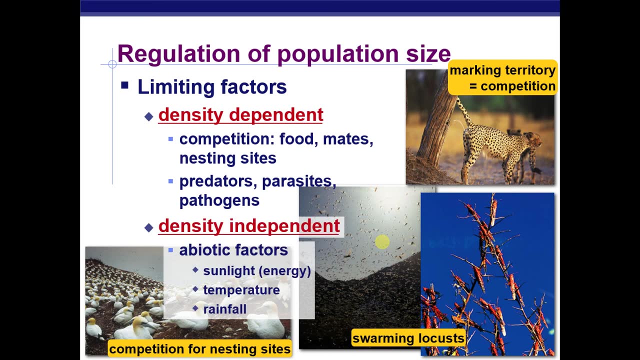 in an oscillation and that's a very common thing to see if we're looking at the population dynamics of predator-prey relationships within a ecosystem. but, like we said, what's key to the exponential growth model is it assumes that are there are limiting factors and there's kind of two types. 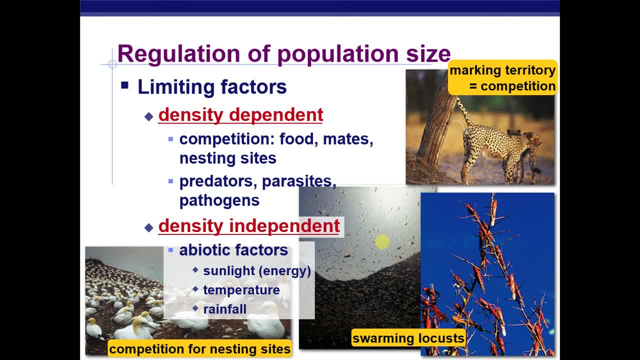 of limiting factors. that we're going to talk about in a little bit, but first we're going to talk about factors. one is called density dependent, where these factors that influence the pop- the size that a population can grow to- are dependent on or their effect is exerted more strongly when there 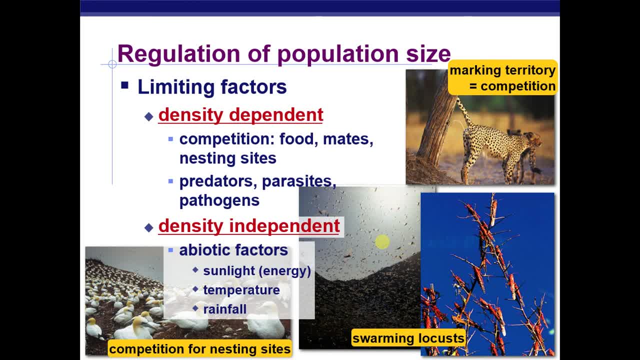 are more individuals than there are less. so competition for food or mates or nesting, predators, parasites, pathogens- all of those are density dependent. they depend on how many organisms they are in that population. the more organisms, the more seriously these factors will impinge population growth. and the smaller the population the set, less seriously they own pinch population growth and then 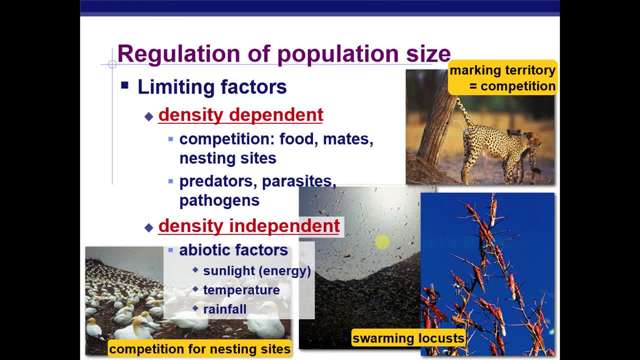 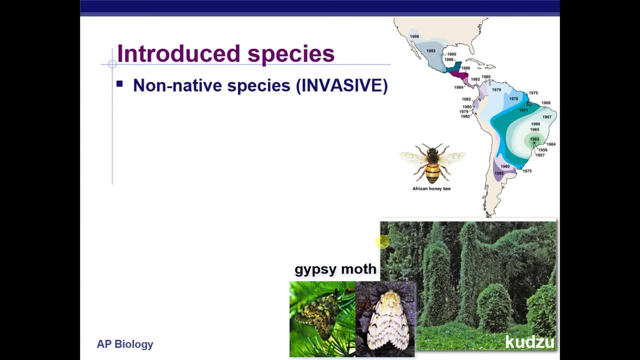 we have what's called density independent factors, which are pretty constant, independent of how many organisms are in a given population. so like rainfall and temperature and sunlight are all examples of those. lastly, we're just going to look briefly at induced species. so these are called non-native species or invasives and they are transplanted populations that are introduced. 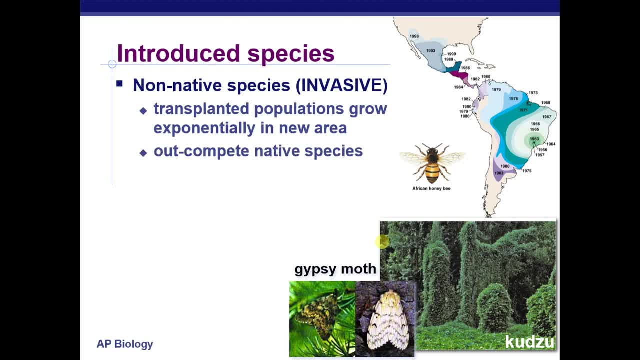 a new area and then grow exponentially in that area because they don't have a lot of natural predators in that environment and so they can all compete a native species and drastically reduce the diversity. so some examples are African honeybees, gypsy moths, kudzu.